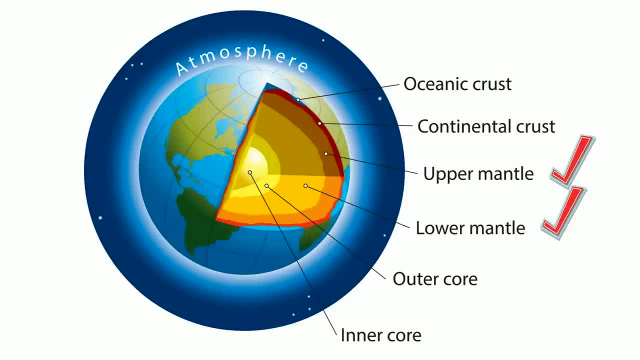 slow-moving solid rock. The mantle is 1,800 miles thick, or 2,900 kilometers, And it's composed of silicate minerals, and they're similar to the ones found in the crust, except with more magnesium and iron and less silicon and aluminum. The core extends from: 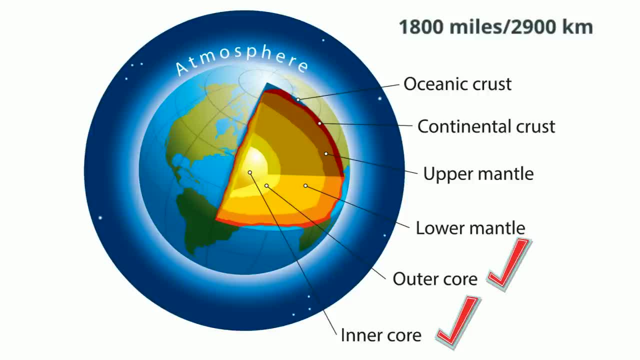 below the mantle to the center of the earth. Scientists believe the core is made mostly of iron and nickel. The core is the densest layer and makes up about one-third of the earth's mass. The outer core is composed mostly of iron and nickel, with metals found in liquid form. 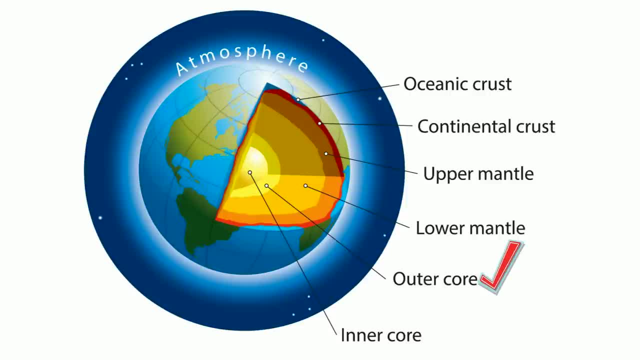 The outer core reaches temperatures of 7,200 to 9,000 degrees Fahrenheit, and it's estimated to be about 1,400 miles thick or 2,300 kilometers. The inner core is the hottest part of our planet and has temperatures between 9,000. 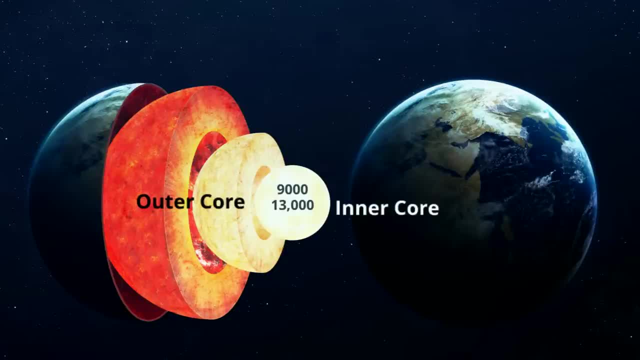 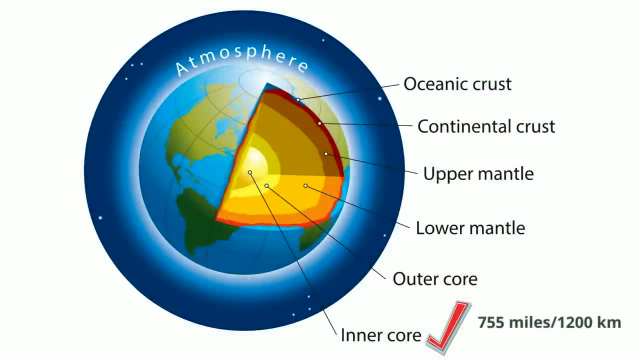 and 13,000 degrees Fahrenheit. It's a solid layer and it's around 755 miles, or 1,200 kilometers, thick, and it's composed mostly of iron. This iron is under so much pressure that it stays as a solid. 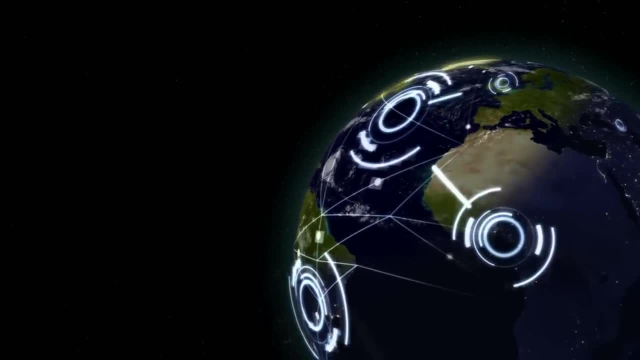 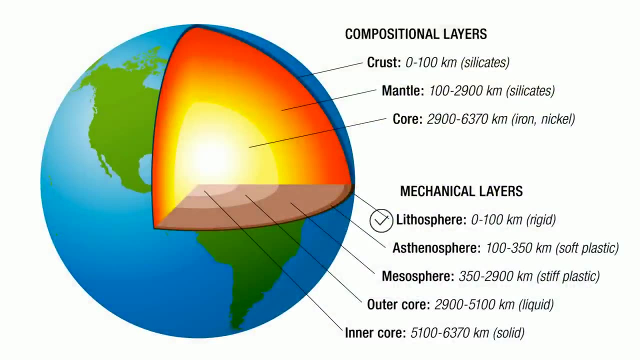 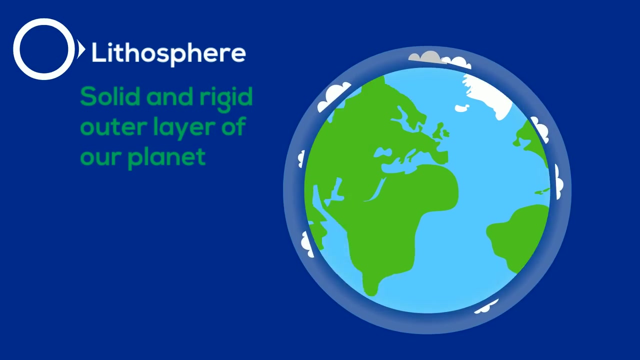 The earth can also be divided into layers based on physical properties, such as whether the layer is solid or liquid. The five physical layers are the lithosphere, asthenosphere, mesosphere, outer core and inner core. The outermost rigid layer of the earth is the lithosphere. 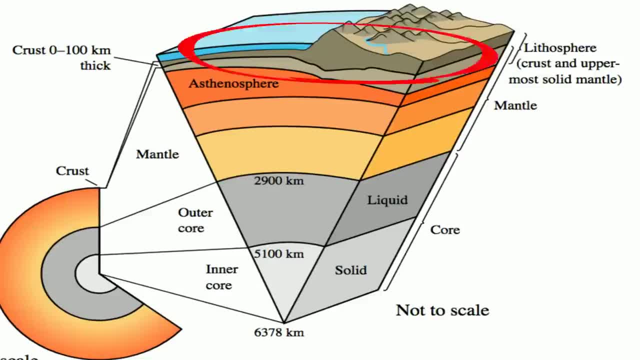 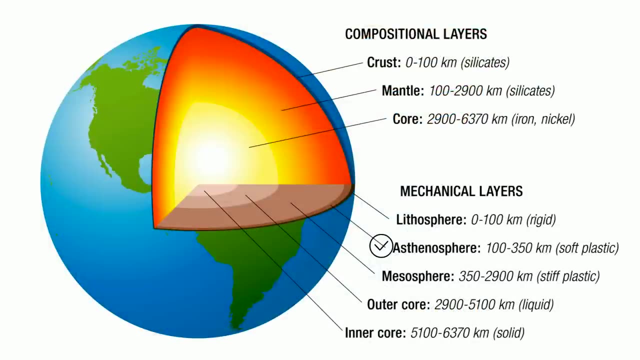 The lithosphere is around 100 kilometers thick and it's divided into tectonic plates. The earth's lithosphere includes the crust and the upper part of the mantle and it is hard and rigid outer layer of the earth. The asthenosphere lies underneath and it's made of solid rock that moves very slowly. 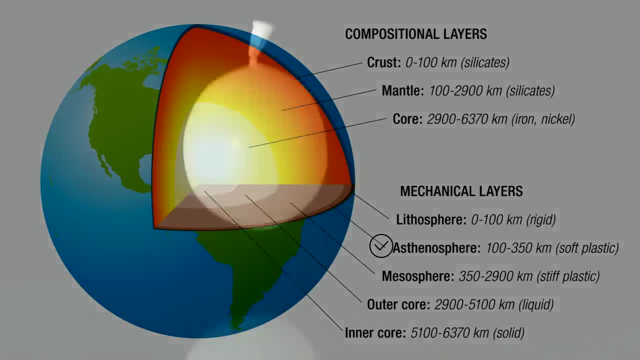 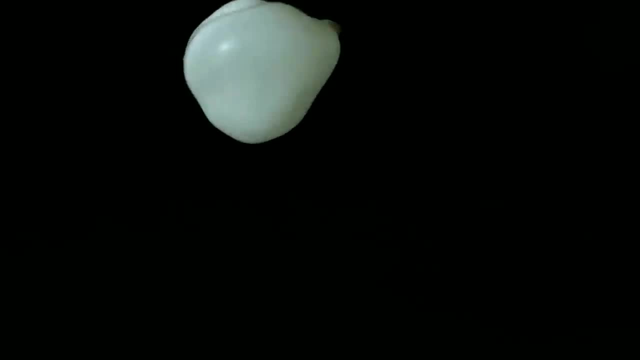 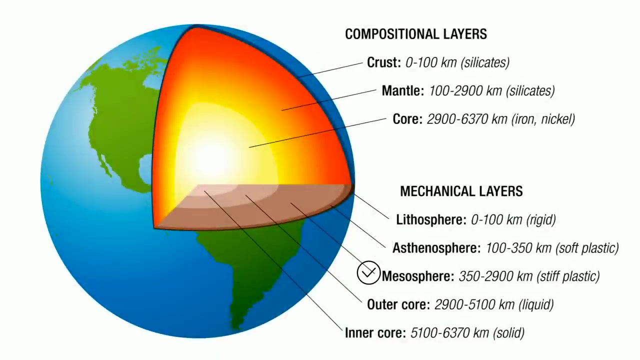 It's described as vissoelastic, which means it can flow and also can be elastic. The asthenosphere is located below the lithosphere and the tectonic plates move on top of the asthenosphere. strong lower part of the mantle is called the mesosphere Rock. in the mesosphere flows more. 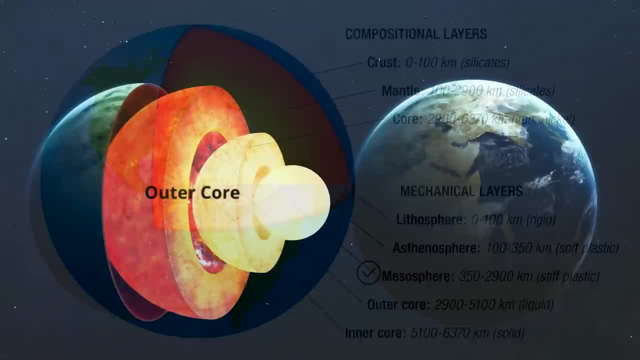 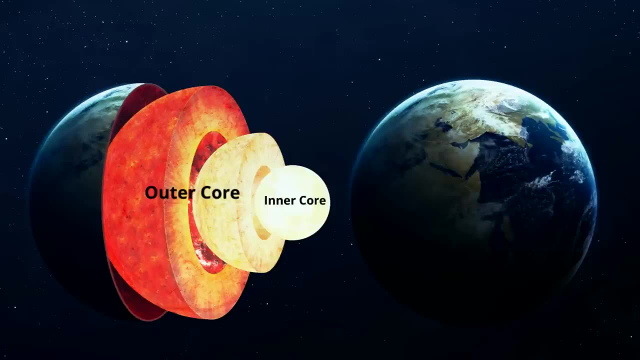 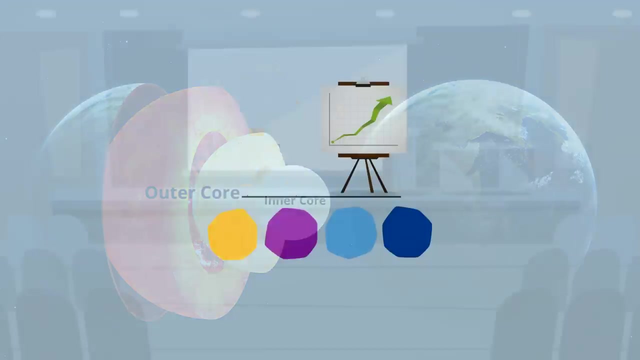 slowly than rock in the asthenosphere. The outer core is the liquid layer of the earth's core and the inner core is the solid part. The inner core extends from the bottom of the outer core to the center of the earth. Thanks for watching. and MooMooMath uploads a new math and science.